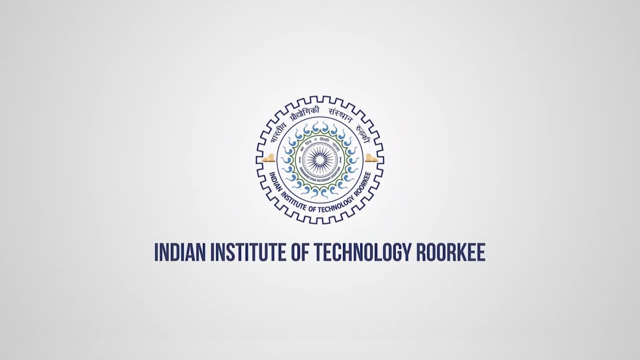 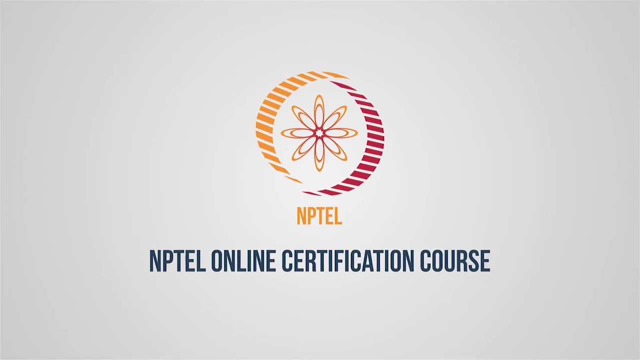 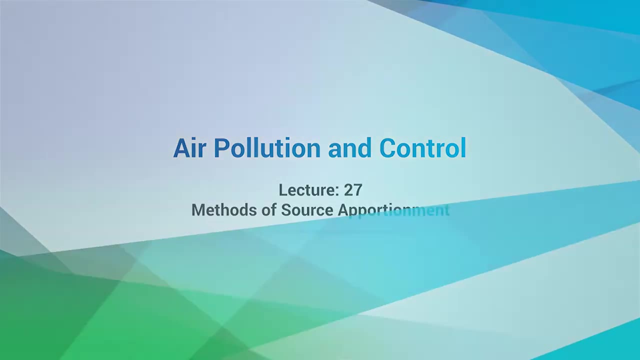 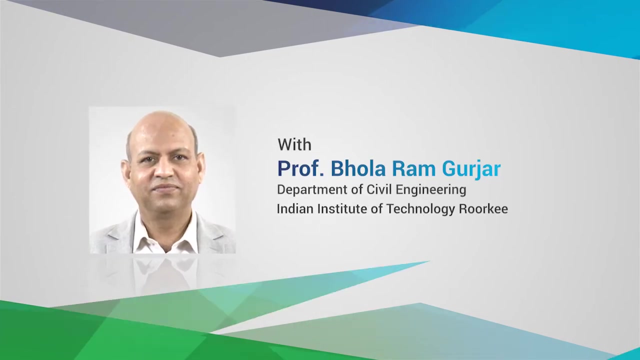 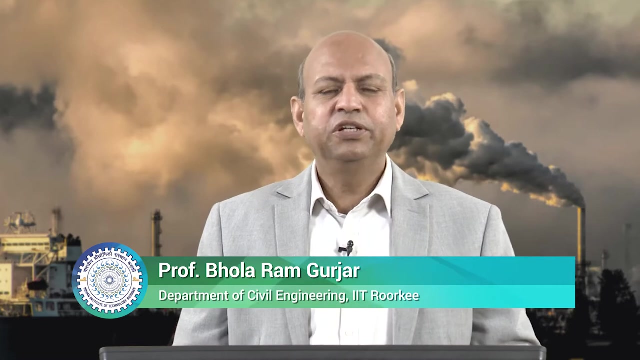 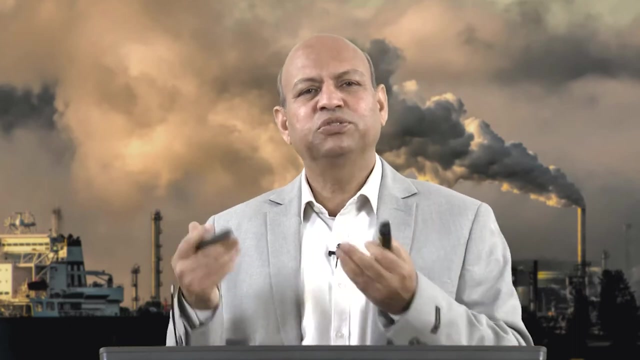 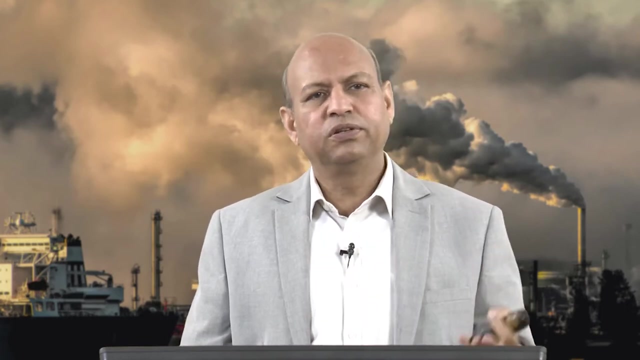 Hello friends, you may recall we have already completed how to develop emission inventory. Today we will start about source apportionment. studies means how to apportion the sources, means different sources of the pollutants and what are different methods for carrying out the source apportionment. So first of all we will discuss about the 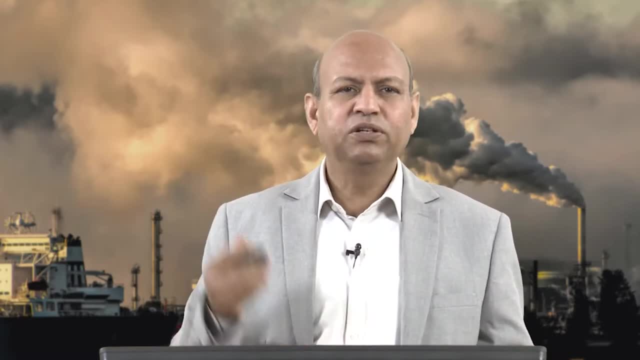 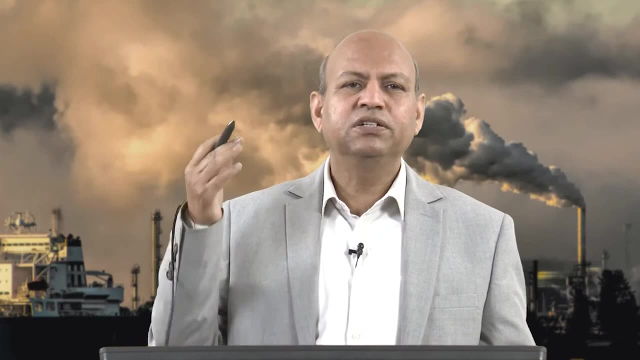 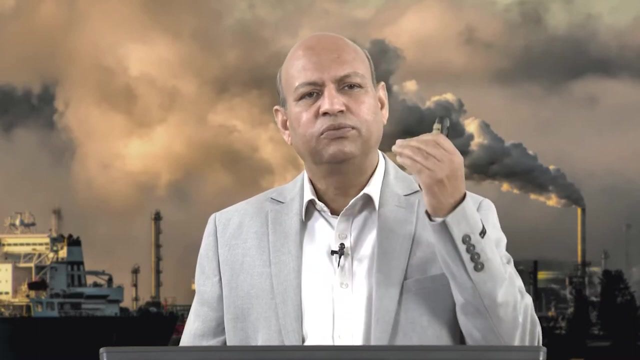 introduction of source apportionment. then we will look into the significance of this particular study which is known as the source apportionment, and then major, you know methodologies like bottom up or source based methods, which are which kind of models we are using for bottom up approach of 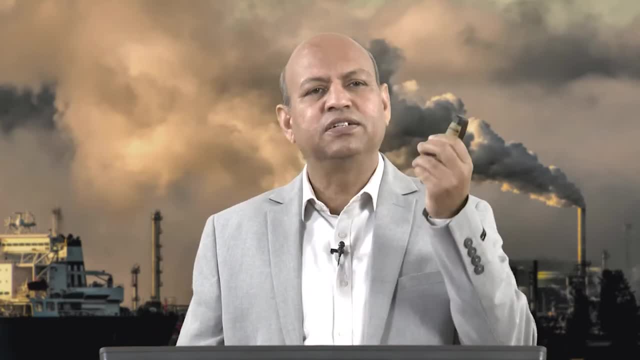 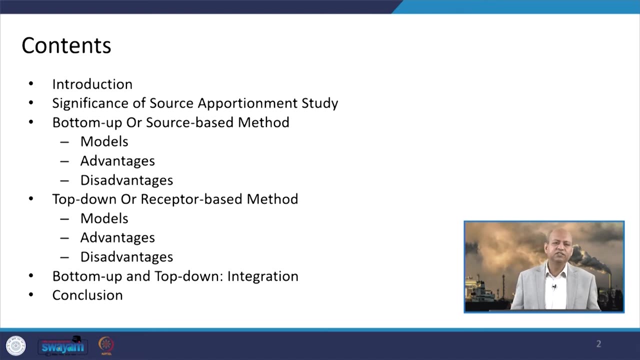 the source apportionment studies and what are their advantages and disadvantages. Then we will look into top down approach or receptor based method models and advantages and disadvantages, and then we will look into the possibilities of integration of both the approaches so that we can have the win-win situation or best features of the both the 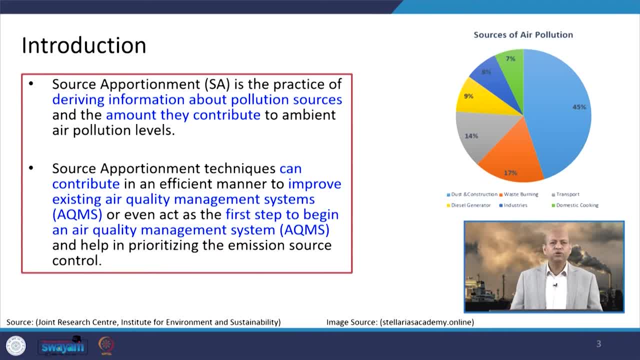 approaches, and then we will conclude. So when we talk about source apportionment. basically this is the you know process or practice for driving information about different pollution sources and the amount they contribute to ambient air environment in terms of different pollution levels. So you can say that this 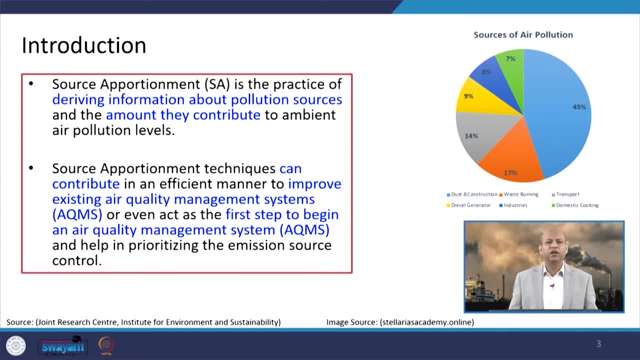 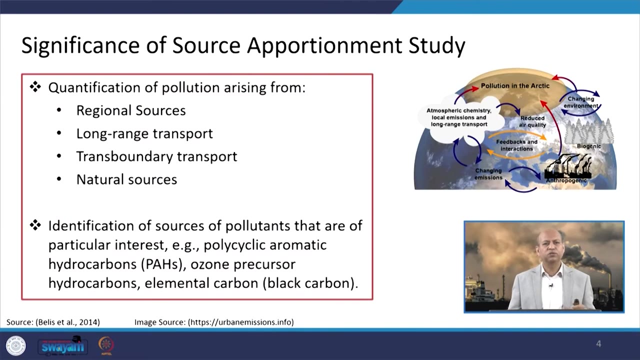 source apportionment techniques. they can contribute in efficient manner of air quality management And they are used in looking into variety of sources which contribute in significant manner so that we can target those sources which are dominating sources, to control the emissions from those sources and then we can reduce the air concentrations of particular. 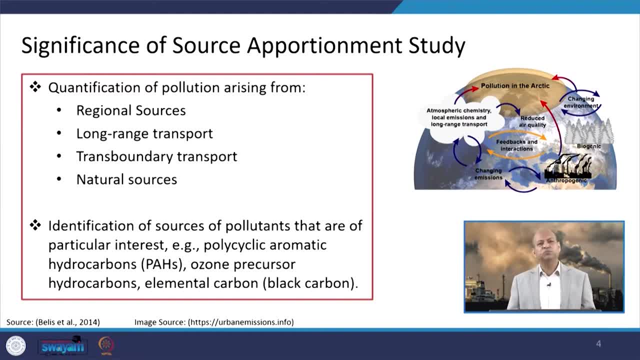 source based emissions. Well, when we talk about significance of source apportionment study, then the quantification of pollutants or the pollutions which are coming from different regions, So the regional sources, or whether it is coming from long range transportation from different areas and transboundary transportation of pollutants also happen- then there may. 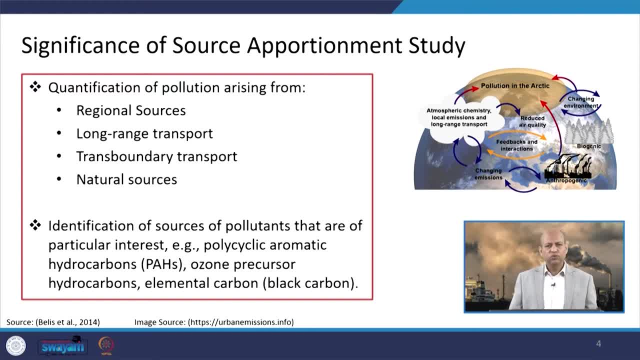 be natural or these anthropogenic sources. So we can really categorize, we can see which pollutant is coming from which particular source in dominating manner. So the identification of different sources, So the specific sources of the pollutants that are of our interest or particular interest. 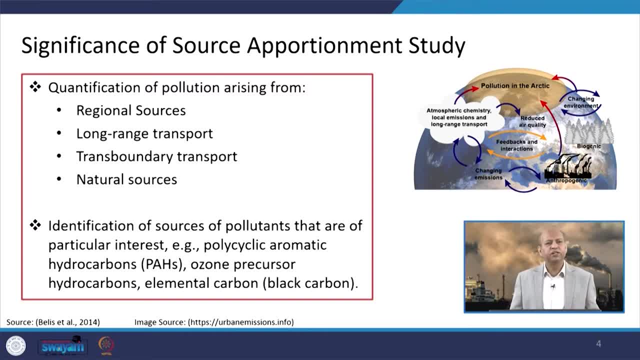 like these polycyclic aromatic hydrocarbons or pH or ozone precursors, like NOx emissions or CO emissions, then hydrocarbons or elemental carbons, black carbons, particulate matters, PM10, PM2.5- all those which are very important from health risk point of view also. 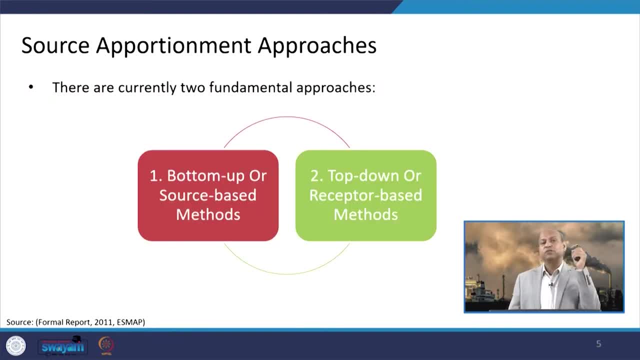 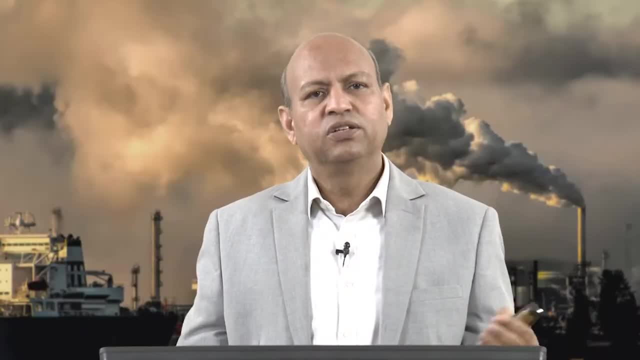 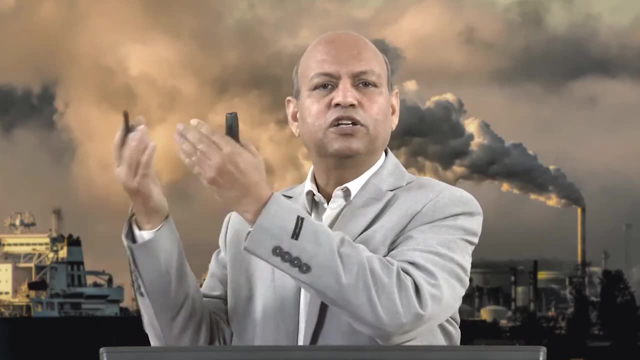 So we look into those pollutants and their specific sources. So the key thing, So the key thing is that a particular pollutant, because in ambient air there are so many pollutants. So if you want to know whether this CO emission or particulate matter emission which has contributed, 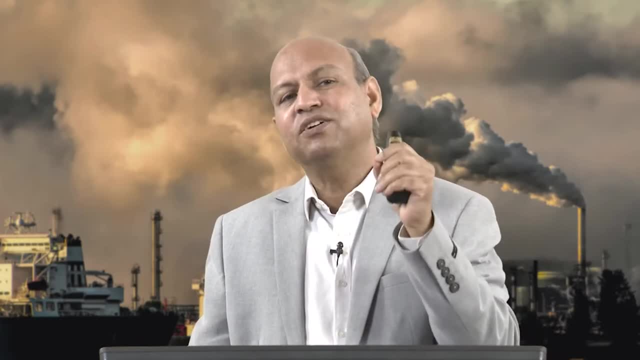 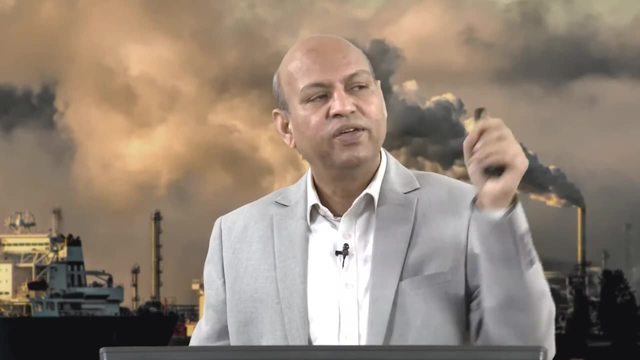 to the air quality degradation, so that PM10 has come from how many sources and what is the amount of that PM10 from different sources, so that we can know that we can list. this is the major source, this is the moderate, this is the minor, so that we can look into. 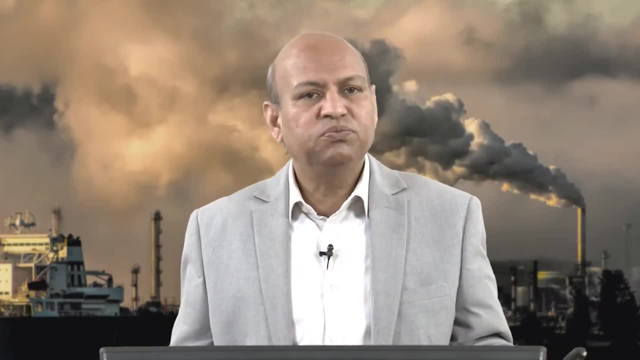 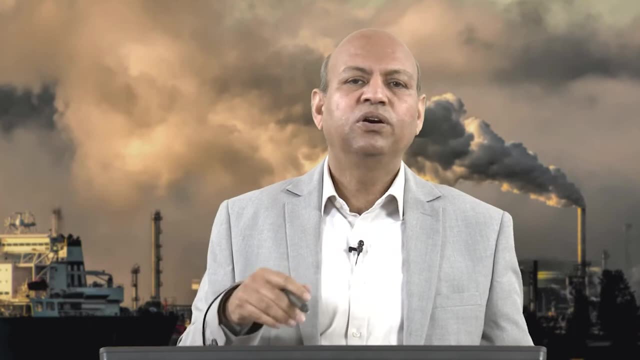 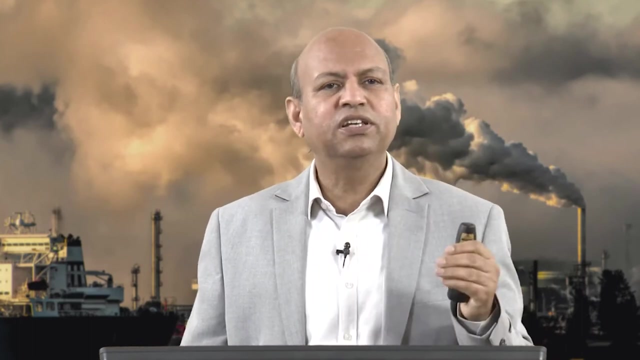 the major sources. basically. Now there are different approaches for doing this: source apportionment, like bottom up or source based approach or method, then top down or receptor based method or approach. So when we look into bottom up or source based method, so basically we focus on the 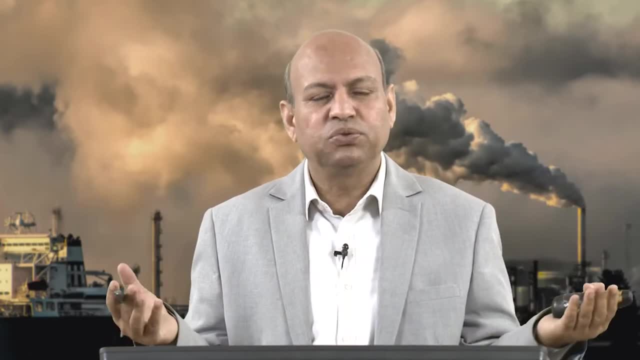 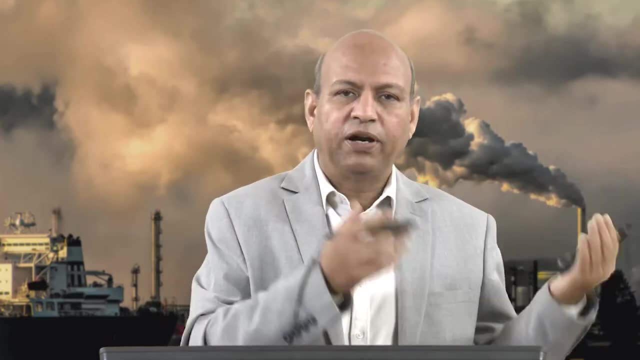 sources. So how many sources are there? which are the major sources like we can have in a town or city? several kind of sources like industrial sources may be there, power plants may be there, or from transportation sector, or domestic sources like and we have to develop emission. 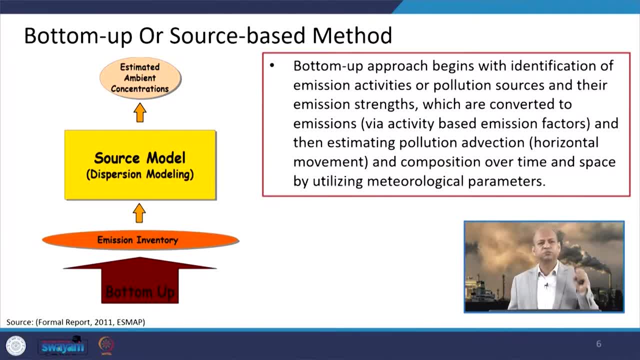 inventory with the specific to the sources basically. So when we talk about the source based methodology of the source apportionment study or bottom up approach, then we are basically talking about emission inventory development and then using the emission inventory into the dispersion modeling. 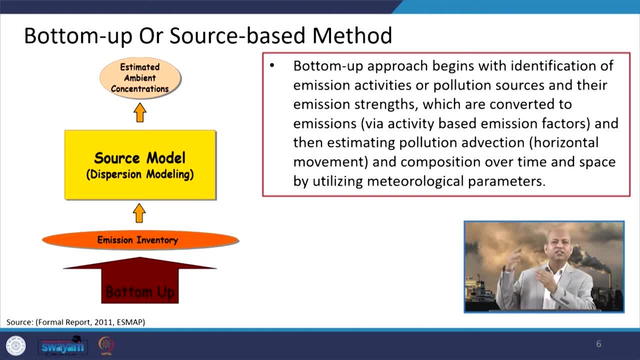 So the dispersion modeling gives us the air quality concentration at certain locations. So that is the bottom up means at the ground level. we need to know how much pollution sources are there, how much pollution is coming from those sources and those pollution, those emissions. 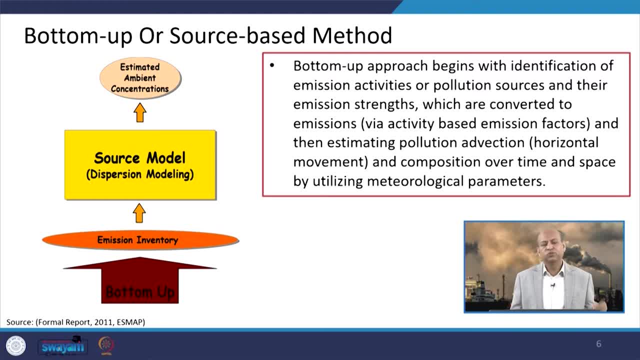 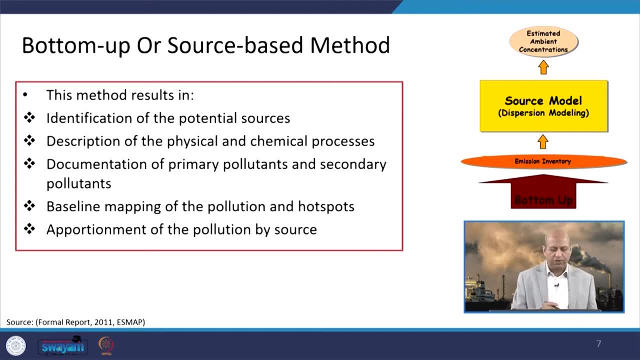 how do they contribute into deteriorating the air quality. so for that we use different dispersion models. So basically, when we talk about bottom up, source based approach, we go into different kind of steps Like identification of the air quality, Identification of the potential sources or important sources. 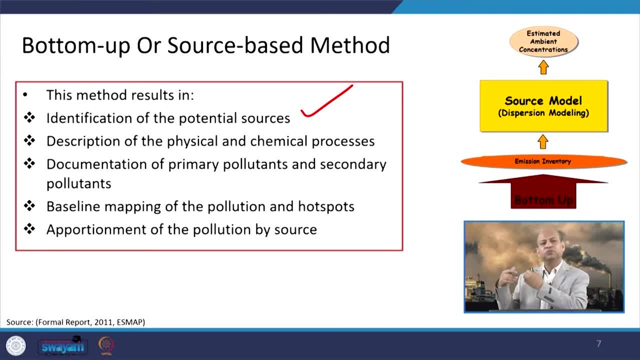 Description of the physical and chemical processes which will contribute into formation of secondary aerosols or pollutants. so we have to document those primary pollutants, secondary pollutants, which are going to be there because of the emissions of different type of pollutants. Then we need to baseline mapping and pollution hot spot pollution levels because, like there, 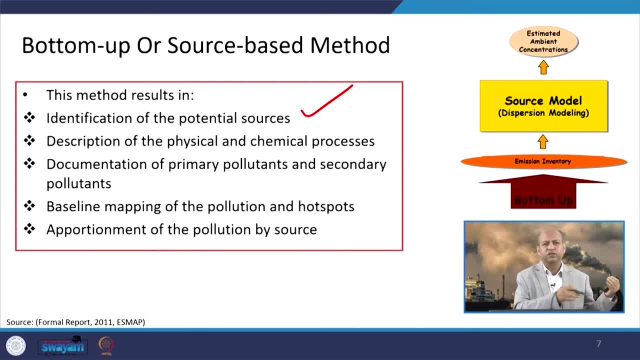 may be some intersection. There may be some intersection of the transportation or highways, so there may be very high emissions of NOx or CO. So we have to categorize or we have to point out that these are the hot spots. or there may be some particular industries in nearby areas. there may be power plants, so maybe 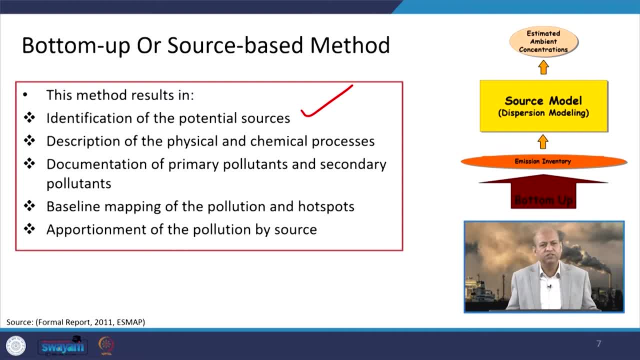 SO2 or particulate matter may be more in those particular places. So we have to identify the hot spots or we have to do the baseline mapping. Then we need to do the apportionment of the pollution by the source using the dispersion modeling. 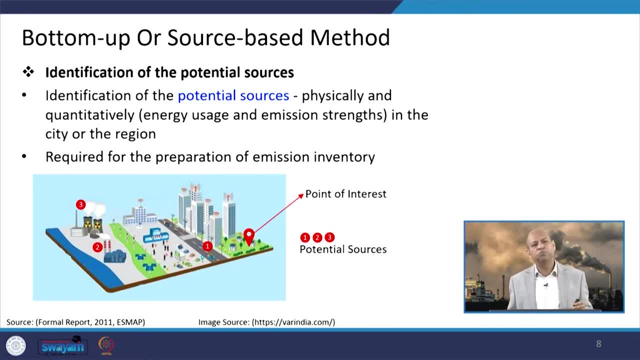 So when we go step by step, when we go for identification of the potential sources, basically we have to look into physically quantification of those different kind of energy uses in industries or domestic sources or sectors, and then their emission strengths, source wise as well as pollutant wise, in the city or particular region of our interest. 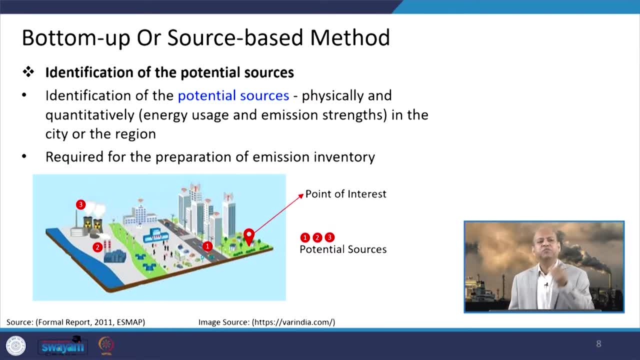 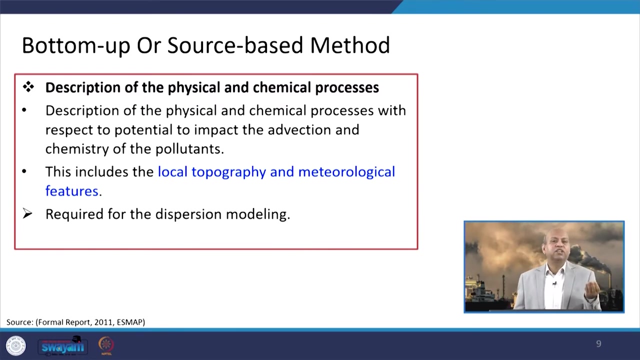 Then we need to go for requirement of the preparation of the emission inventory, because without emission inventory 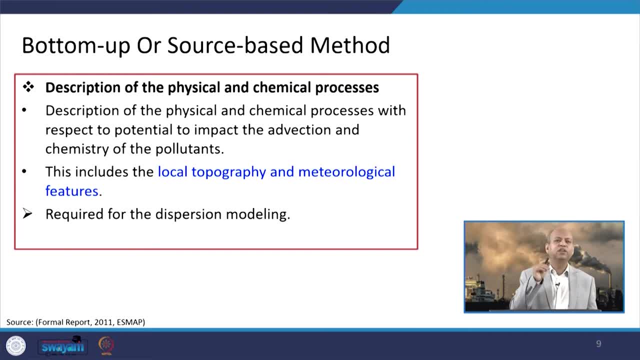 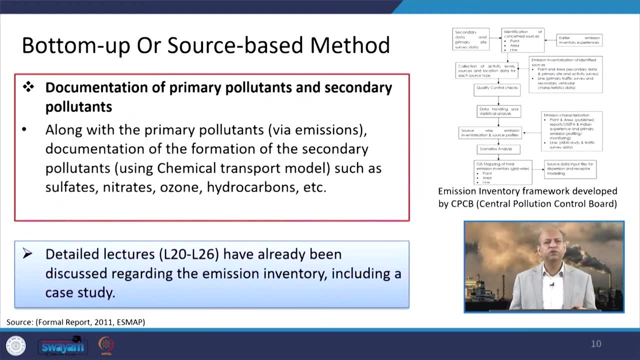 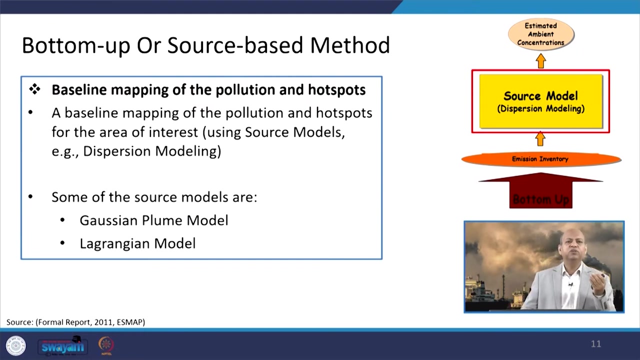 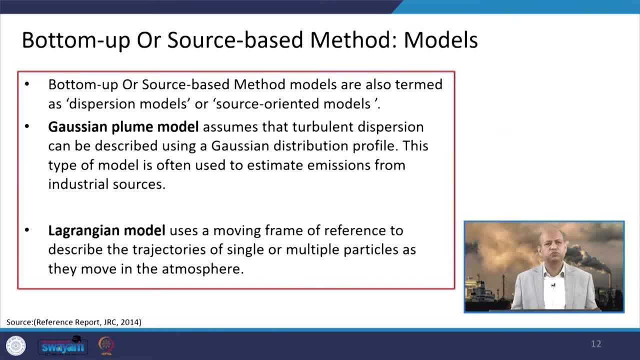 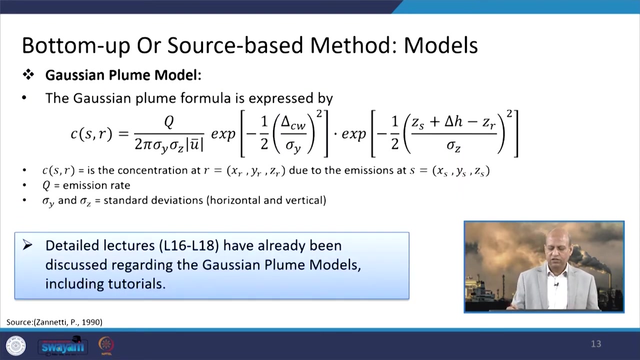 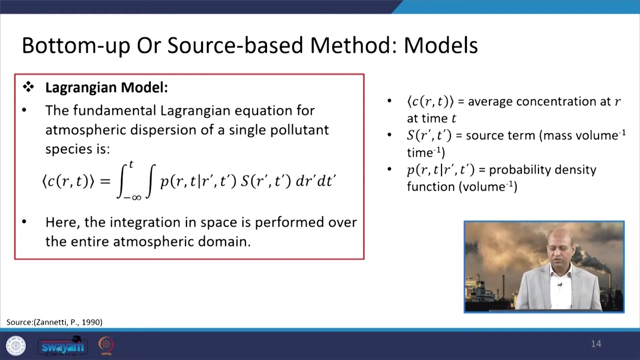 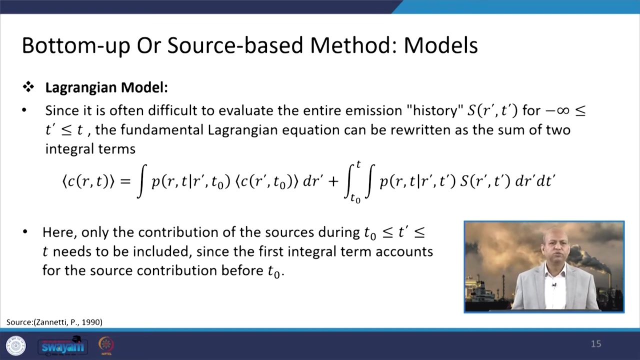 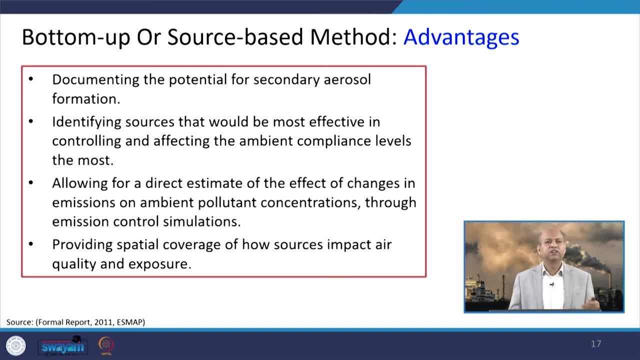 So we can identify those particular sources and we can directly estimate the effects of those changes in terms of emissions and in terms of ambient air quality concentration, plus spatial variation, temporal variation, those kinds of things of the air quality and exposure we can do in this particular activity of the bottom-up approach. 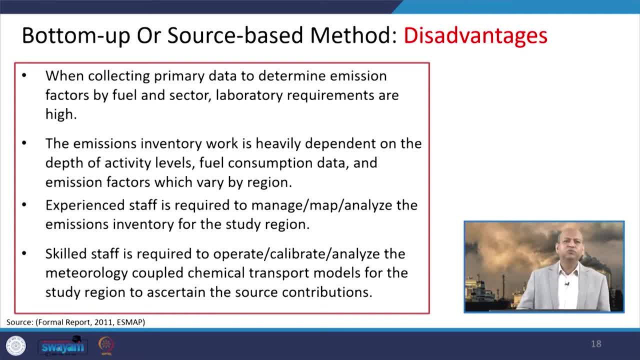 But there are certain disadvantages also, like when we go for collection of primary data and we go for emission inventory. development based on emission factors and laboratory requirements for those generating those emission factors is very expensive process, basically Highly complicated laboratory equipments we need for, like, different kind of vehicle emission. 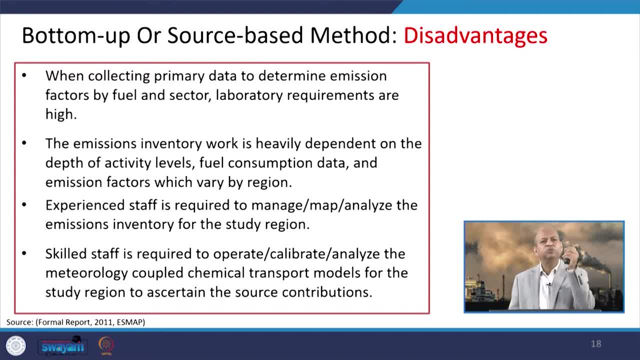 factors. So for each activity, if we need to have the emission factor, it is a huge task, basically needs lot of resources, lot of infrastructure. Similarly, for development of emission inventory we are heavily dependent upon those activity level data, fuel consumption data. so uncertainty may be there and it can vary from region to 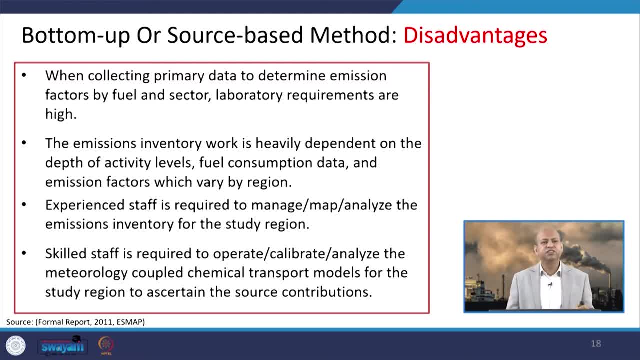 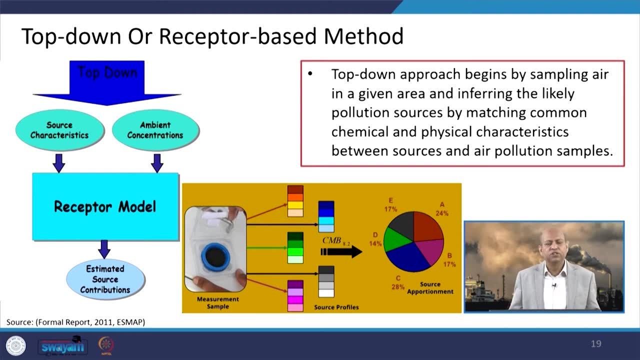 region and then experienced or skilled staff is needed for developing emission inventory, for calibrating the emission estimating tools or models, plus dispersion models, Now if you go for top-down. So, for example, if you go for top-down or receptor based approach method, which is another- 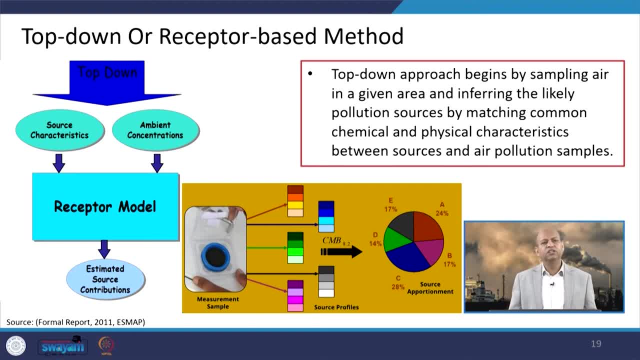 very popular method which we will see. So in this. basically we go like for sampling, we go for the air quality concentration sampling and then we match those air pollutants concentrations to the pollution sources, because we also identify the pollution sources. So different markers are there, there are different signatory pollutants from different 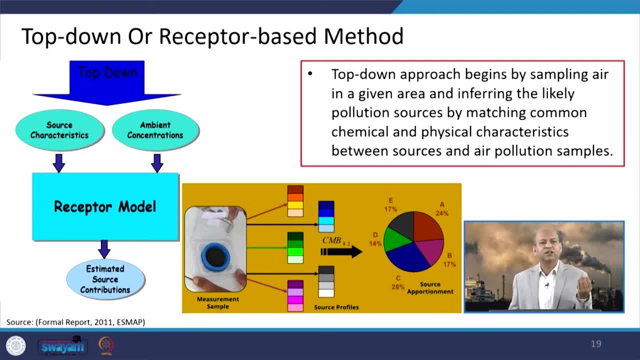 sources, Like, as I said in one lecture, That if you are given a table and in that table you see the NOx emissions, NOx concentration is very high or CO concentration is very high, So you will intuitively think that this site may be near to the transportation sector. or 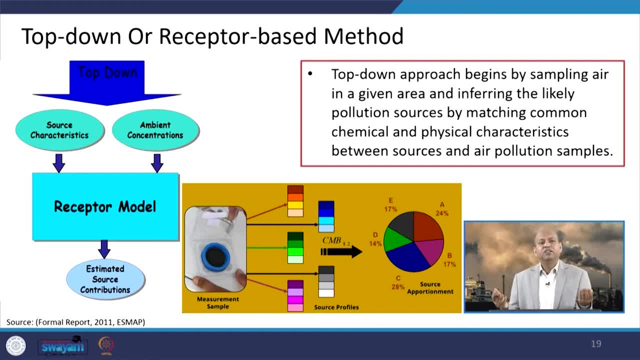 some highway or something like that. If you get high concentration of SO2, etcetera, then you may assume that maybe coal based thermal power plant is nearby. So that way you can link, you can match, basically, and there are statistical tools also. 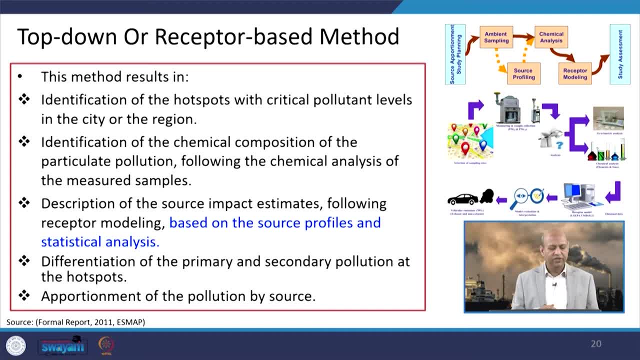 So we will see In this particular top-down approach. basically we need to identify first of all the hot spots of the pollution sources and the levels, as we do mapping through air quality monitoring and the identification of the sources. Then we go for identification of chemical compositions of different particulate pollution. 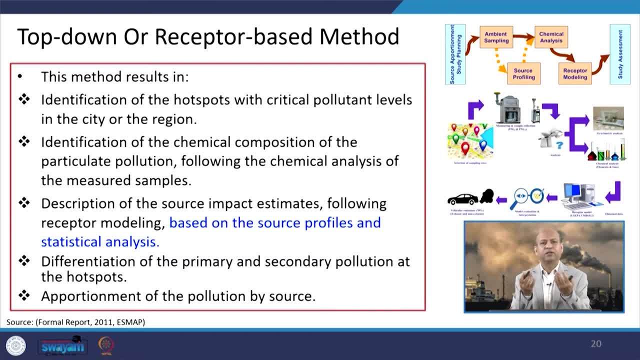 Chemical analysis is to be done after. when you collect particulate matter, then you go for chemical analysis in the laboratory. So you know how much heavy metal is present in that particulate, What is the particulate matter or which kind of different pollutants are present there. 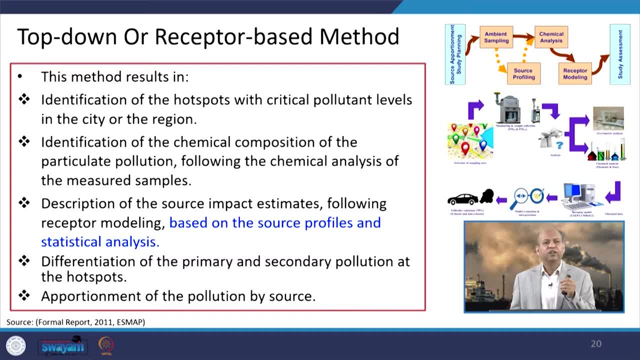 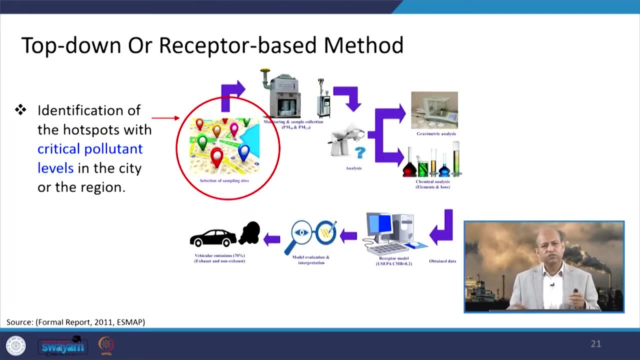 Well then we describe, based on the source profile and the statistical analysis we have to do. So we can basically match the sources and the pollutants and we can differentiate between primary and secondary pollution also, And then we do the detailed apportionment of the pollution with respect to the source. 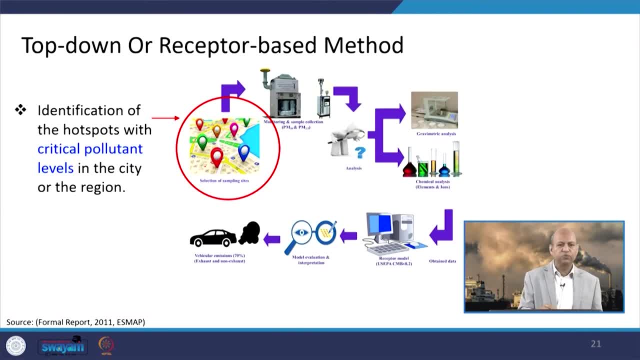 Basically, when we go for these identification of sources, Then monitoring of the pollution, Then we go for the identification of the sources, pollutants, and then we go for this chemical analysis, and then we go for this matching of the statistical tool, utilization for apportionment. 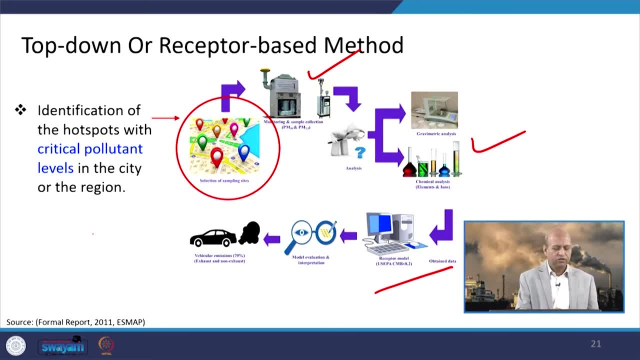 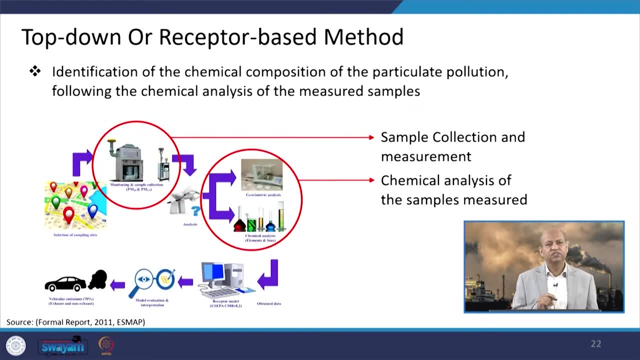 So all these are, you know, given in this particular picture. So the first of all, the critical pollutant levels have to be identified, those locations where lot of pollution is there, right? The second is identifying the chemical composition of the particulate pollution. okay, 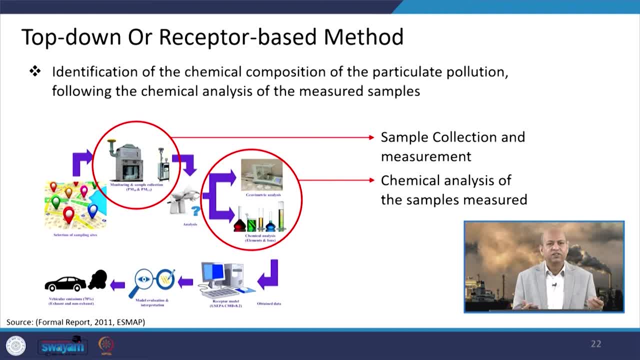 So for that we have to do chemical analysis in the laboratory, basically So sample collection, and then the measurement of those samples and take to the laboratory for chemical analysis So that we can know several kind of pollutants, which are toxic chemicals, available in those. 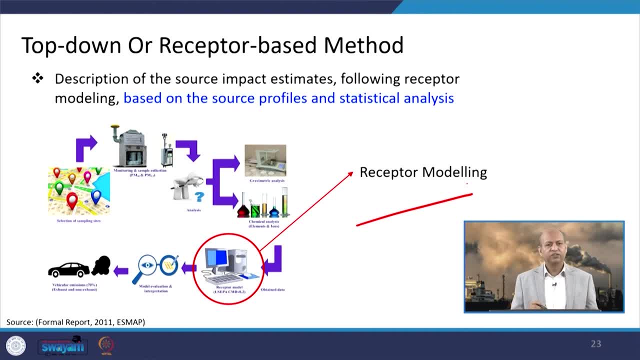 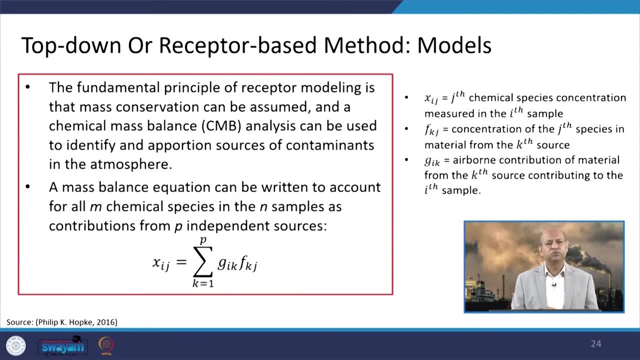 particulate pollutants. Then we go for this receptor modeling, So like chemical mass balance or PMF, etc. we will see later on. So those kind of tools we will basically use, okay. So like, as I said, that the fundamental principle of the receptor modeling is basically the 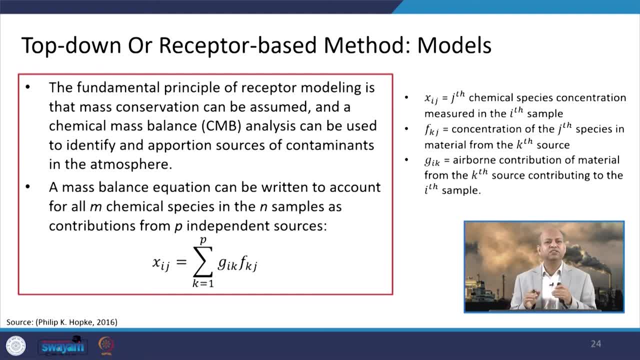 mass conservation. So the chemical mass balance analysis can be used to identify and apportion the sources of the contaminants in the atmosphere using the CMB technique basically. So mass balance equation which is used for this particular purpose is this one. You can see the chemical species of different nature, i-th or z-th. okay, 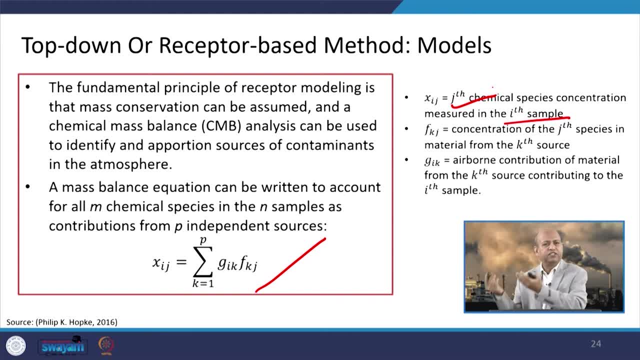 In i-th sample z-th. chemical species can be mean different samples may be there, different species may be there. So we represent like that Then the concentration of that particular species in the material form okay from the k-th source right and then airborne contribution of those particular material from the k-th. 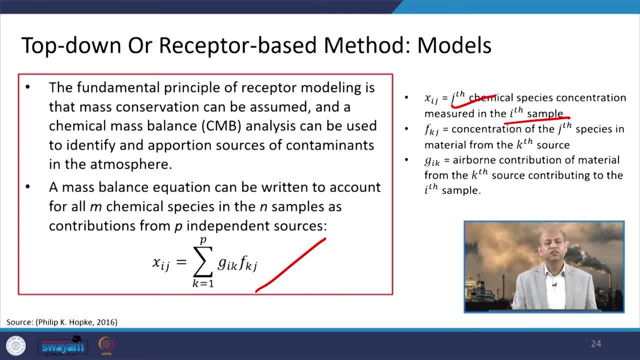 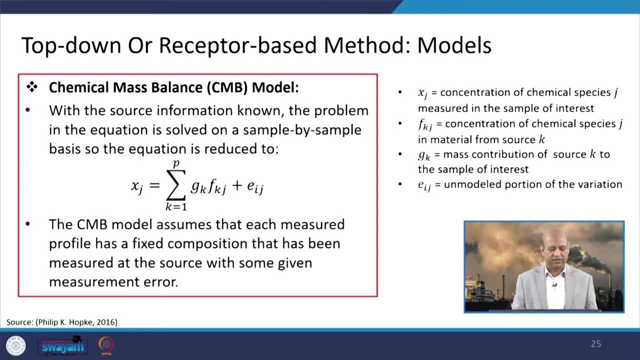 source contributing to the sample. So their relationship is, you know, expressed with this particular equation and this you know equation, further simplified as a CMB model, in this particular form, So that you can easily calculate which kind of species coming from the sample. 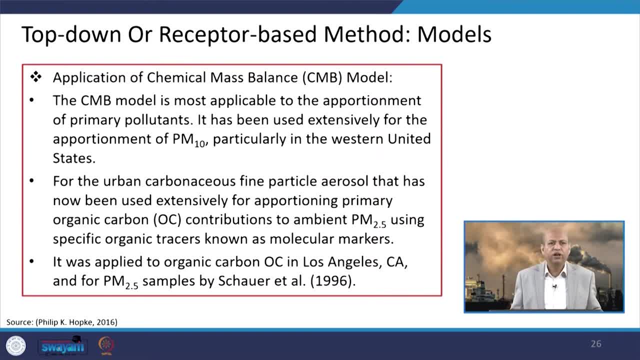 Which kind of specific source? Well, so when we go for this top down or receptor based modeling, that is, the CMB modeling, or chemical mass balance modeling, basically. So, for example, we go for PM10 apportionment. So in PM10 you know whether elemental carbon, organic carbon or some heavy metals are present. 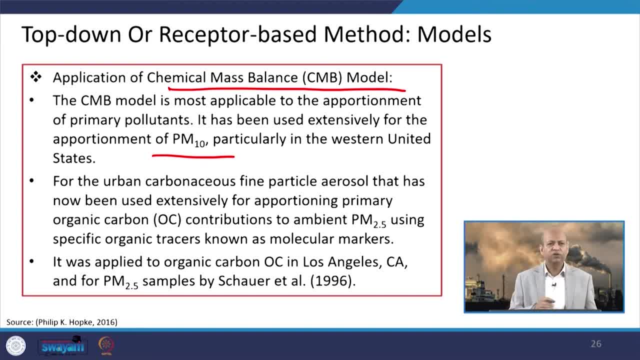 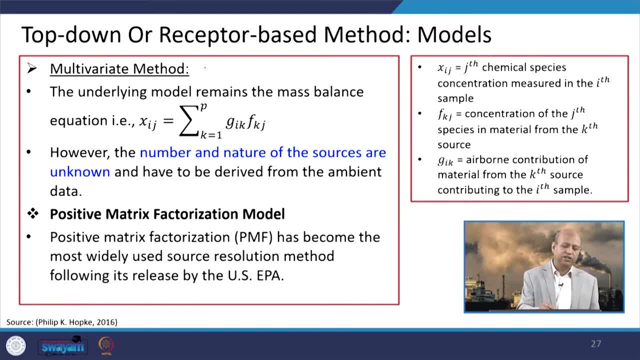 or carbonaceous fine particles are there For that. it is, quite you know, usable for using the CMB technique. Then there is another method, that is the multivariate method. okay, and in under that multivariate method, basically you can use this positive matrix factorization model, or PMF, that is. 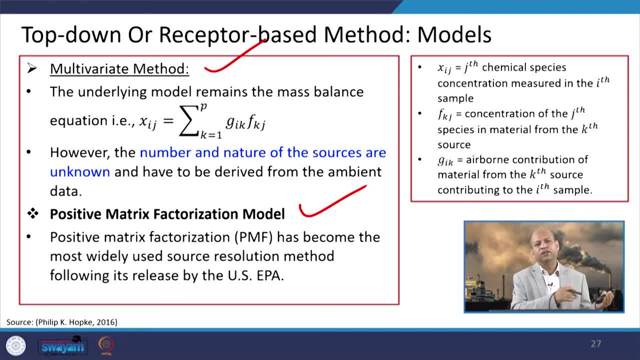 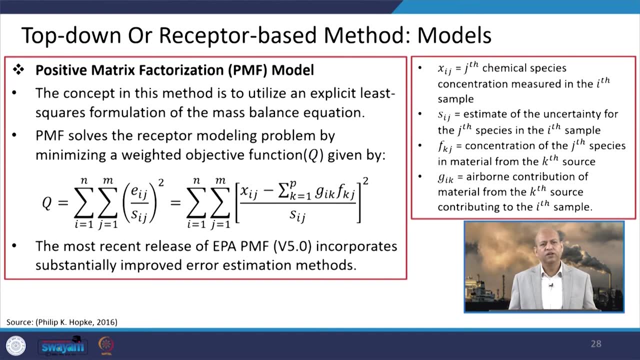 very easy tool and that can relate the pollutant with the specific source and this is, you know, computer based technique and statistical analysis is to be done and USEPA has, you know, used it, that it has been very popular among atmospheric researchers or air quality scientists. 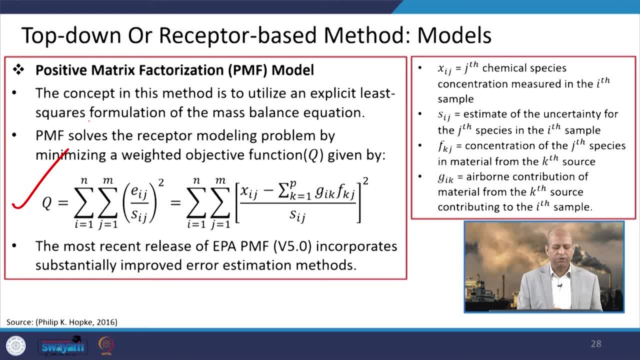 So this is particular relationship which represent this PMF model which can be used like chemical species. then uncertainties may be there. concentration of that particular jth species- again the same concept, airborne contribution from particular source. So all those you know IJK, whether it is you know species or that sample, or the source, 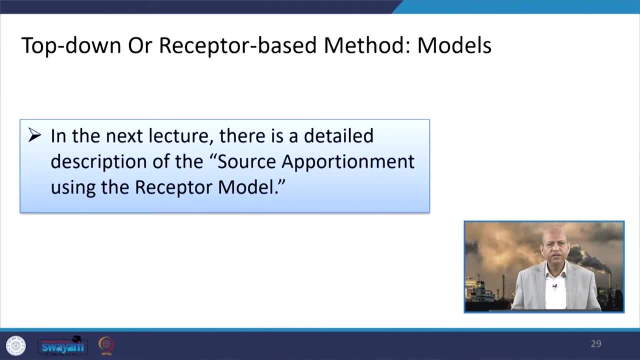 that has to be related with the each other. So this particular, you know, top down or receptor based model or method in the next lecture we will discuss in detail, So we can just skip at present the source apportionment using the receptor model. 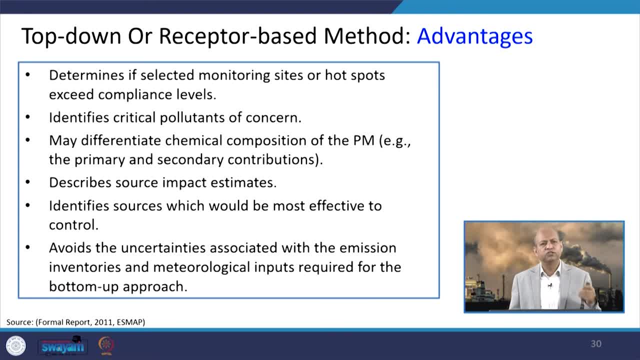 So we can directly come to what are the advantages and disadvantages of the receptor based method. Basically, it can determine those monitoring at the selected monitoring sites, hot spots, some particular, you know, compliance levels, whether it is exceeding or meeting the those air quality standards or not. 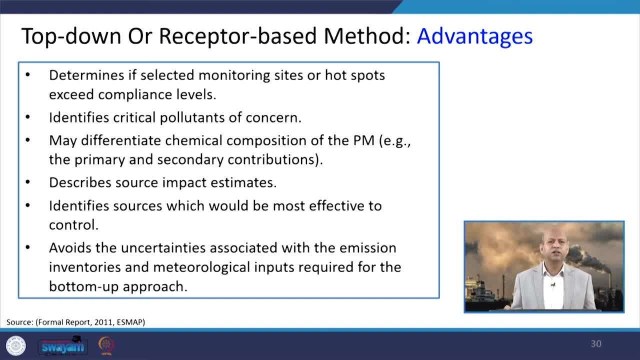 It can also help us in identification of those critical pollutants of the concern which can have severe health effects, etcetera. It can also be used for differentiating chemical composition of particulate matter in terms of primary or secondary contributions. how much is there Then? description of you know source impact estimates can be done by this JIT. 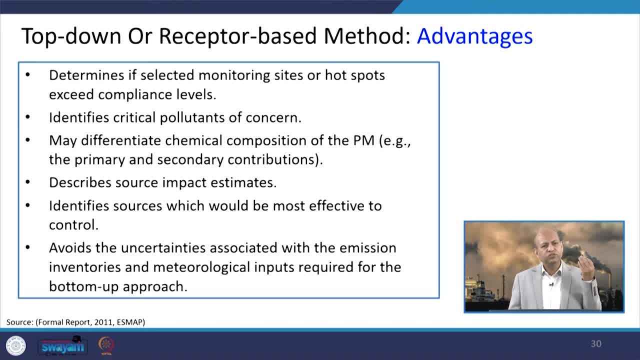 Okay, So this is the technique: receptor based model Identification of sources with respect to the most effective controlling technique. because when we know the dominating source we can judge what kind of technology we can use to control that particular source And it can also avoid some uncertainties which are quite part of that emission inventory. 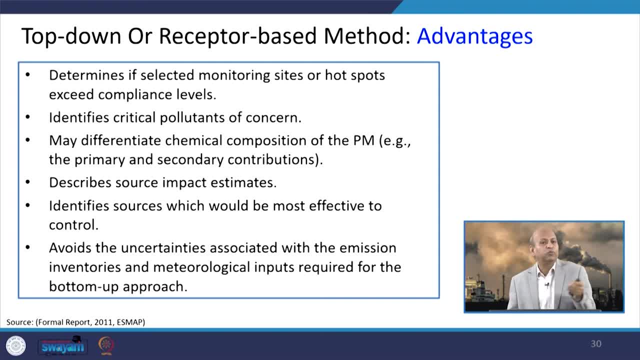 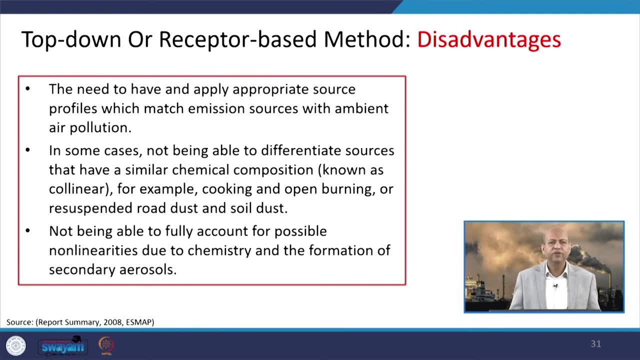 based modeling or the bottom up approach, So that kind of uncertainty can be reduced and it is much simpler and much cost effective In terms of resources and skilled manpower. Then there are certain disadvantages also like it needs to have and apply appropriate source profile which can match emission sources with the ambient air pollution, which is you. 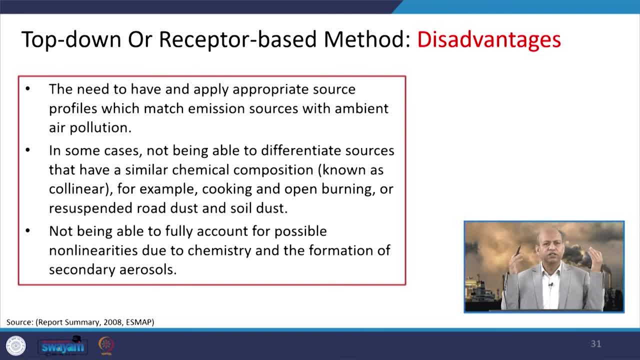 know. again, it is not so easy. it needs some intuitive gas as well as some laboratory based analysis. those kind of things we need to know and the computer modeling- skilled manpower is needed. So in some cases you know not being able to differentiate between the sources that can. 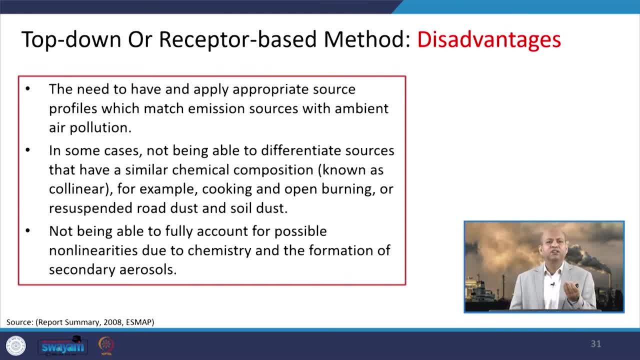 have similar chemical compositions. For example, like you know, cooking and open burning will have similar kind of air quality pollutants. So it is difficult whether it is coming from the- you know- open burning or from the cooking. Otherwise in emission inventory we can have, you know, different emissions. 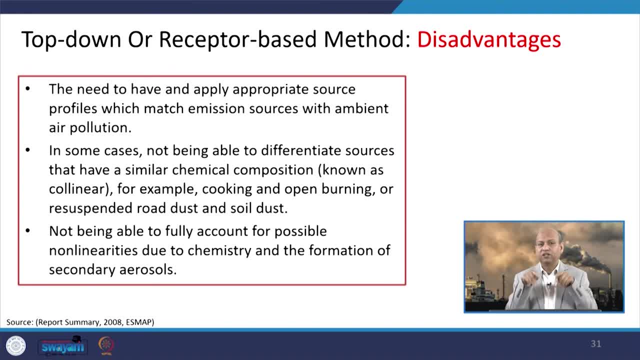 So that is the advantage in that bottom up approach, but in top down this is the limitation, because we cannot differentiate In terms of those particular pollutants which are common in both the sources right, like road dust and soil dust can be simple. So it is coming from the resuspension of the road dust or from the soil dust we do. 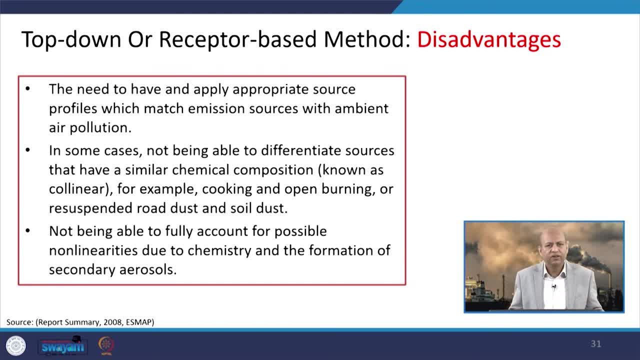 not know. So that is the limitation in this particular approach. Also, you know, it is not possible to be able to fully account the possible, you know, non linearities due to the chemistry and the formation of secondary aerosols, Because that is one more issue. 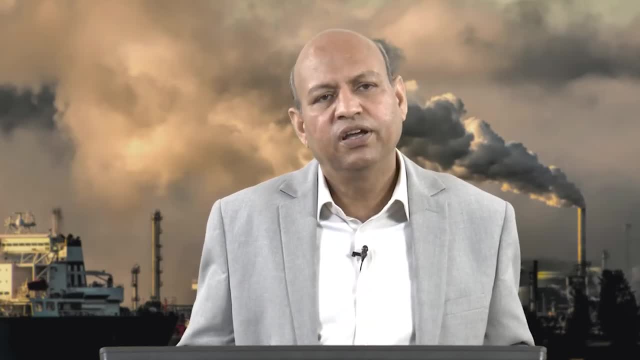 So it is not possible to be able to fully account the possible non linearities due to the chemistry and the formation of secondary aerosols. So that is one more limitation in this particular approach. But now we talk about the integration of the bottom up and top down approach, because both 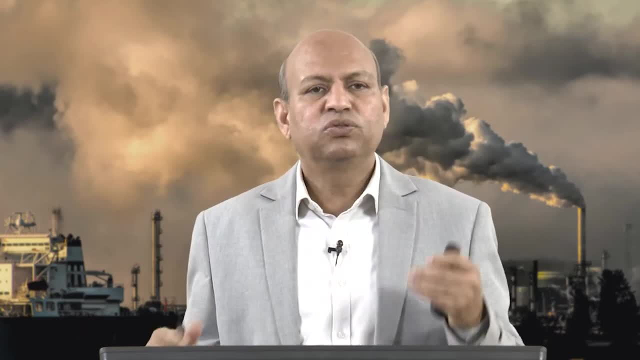 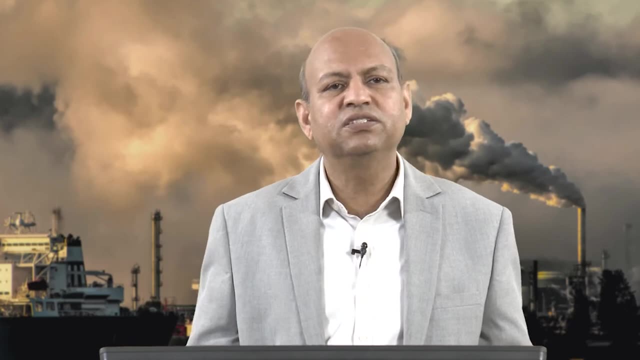 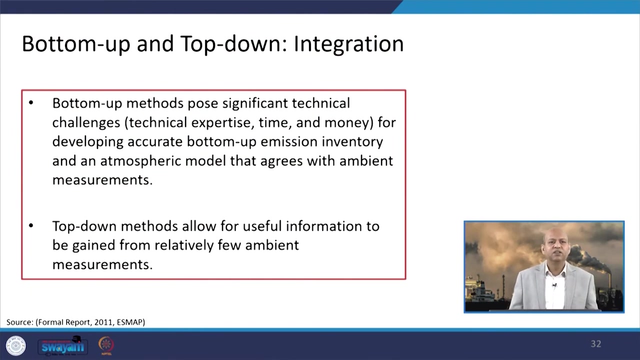 have certain advantages, both have certain limitations. So if we get those advantages, you know, integrated, then we can have better kind of analysis and better kind of results. So the like bottom up approach, which you know give the technical challenges or like in terms of time, in terms of resources, etc. various kind of advantages. 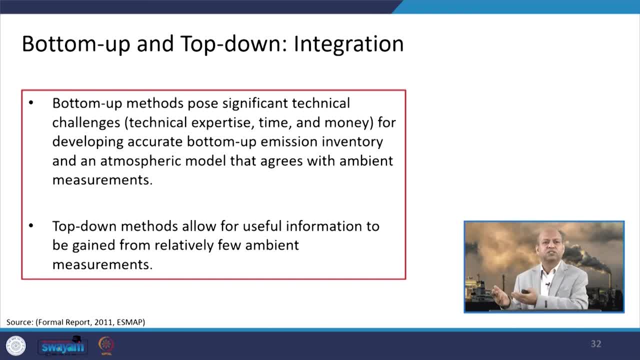 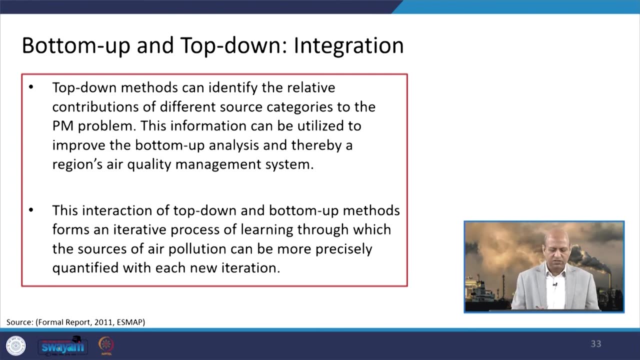 So if we get those advantages, then we can have better kind of analysis and better kind of results. So where is you know? this top down approach is quite simple in terms of very few resources are needed, So that way you, we can integrate those approaches where. so you know, we can look into these information. 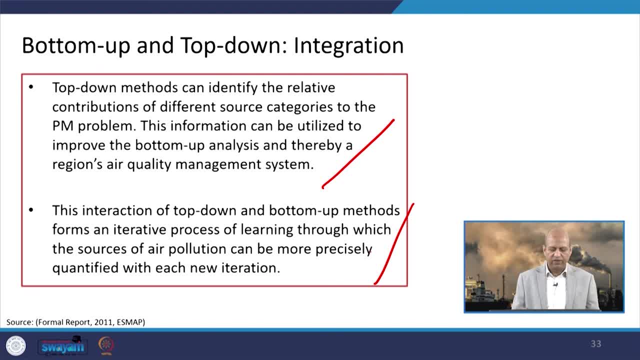 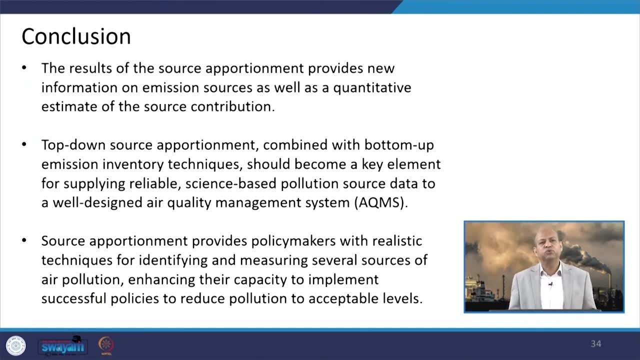 which are available through bottom up or through the top down, and we can have the best aspects of the both the techniques and we can, you know, that way, minimize the limitations of both the approaches. So, in conclusion, we can say that the results of this source apportionment provides new information. 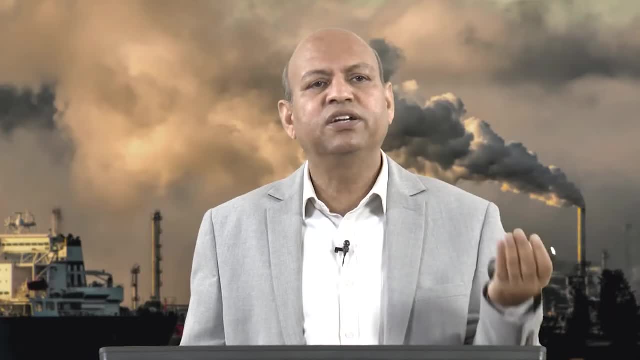 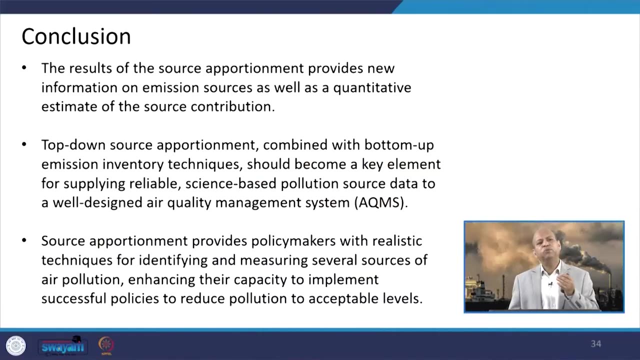 in terms of emission sources, as well as it gives us the quantities of different estimations of source specific pollutants. okay, Then top down source apportionment combined with bottom up. when we integrate that approach, like emission inventory techniques, as well as you know PMF technique, etc. it gives us 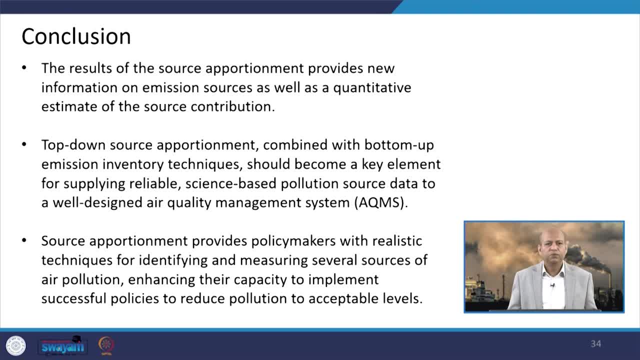 much better results for air quality management. Okay, management systems Plus source apportionment provides policy makers with realistic techniques and information so that we can go for targeting only those sources which are more dominating and which are like low hanging fruit, so that air quality improvements are quite quick. 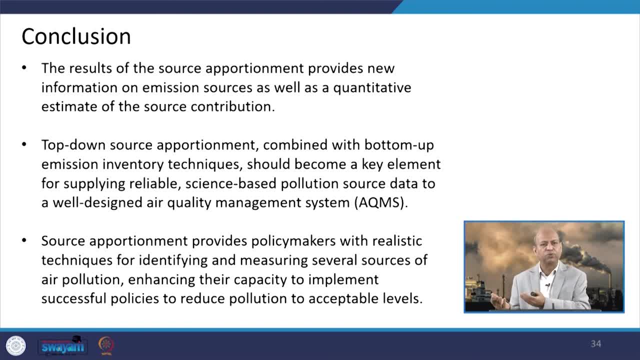 If we do not know the specific sources which are contributing to a particular pollutant, then it is very difficult to make a policy or to make a program to reduce those pollutions. So that way, source apportionment is very important because it gives us an idea which particular